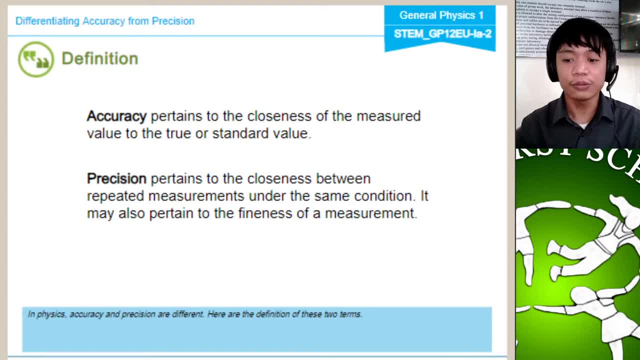 So let's proceed. So in physics, accuracy and precision are different. Accuracy pertains to the closeness of the measured value to the true or standard value. So when we say accuracy, so mas malapit siya sa totoong value, Halimbawa, mas malapit siya sa bullseye. kung pinag-uusapan natin dito is yung dark board, okay, or yung dark game. 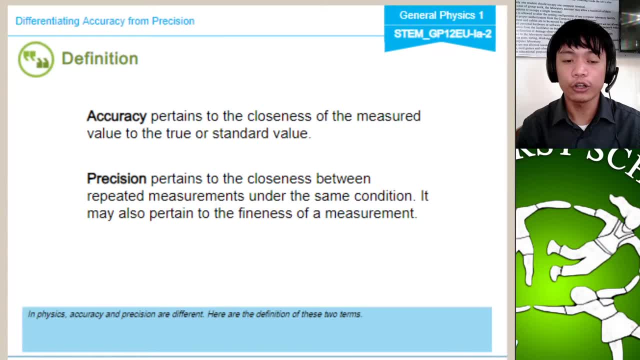 Yung dark sa or yung mas malapit mong matamaan yung bullseye. okay, What about precision? So when we say precision, it pertains to the closeness between repeated measurements under the same condition, and it may also pertain to the fineness of the measurement. 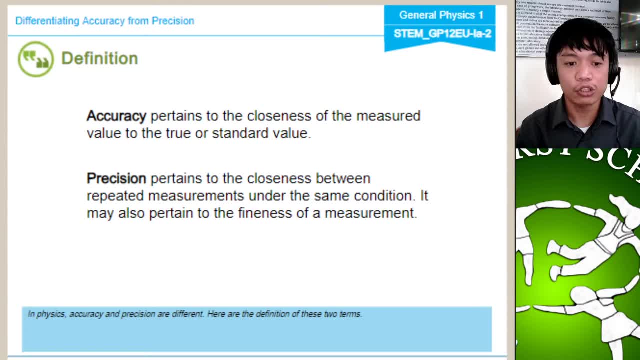 So nandito na mismo yung kanyang definition. So what do you think? repeated measurements? So there are different repeated measurements. So halimbawa, ikaw nag-player, baulit-ulit mong tinamaan yung board, So it is a repeated measurement. 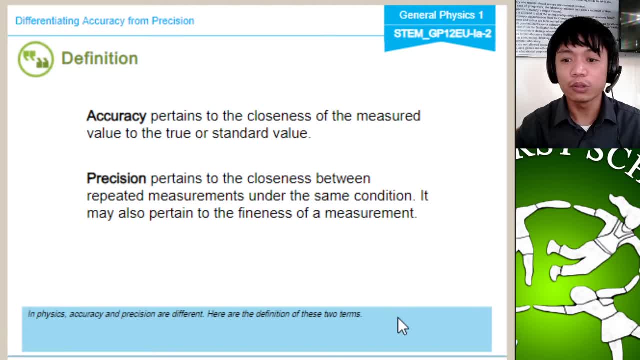 Yung, gusto mo, gusto mo kasi tamaan yung bullseye. So meaning to say you have a repeated measurement But it pertains to the closeness, sabi niya. So parang magkakasama yung mga repeated measurements. 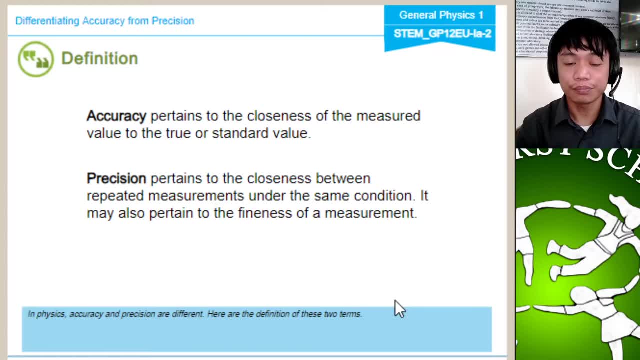 Yung repeated measurement na yun in a particular, in a particular aspect, parang ganon okay. So when we say accuracy pertains to the closeness of measured value, So when we say precision, closeness between repeated measurements. So take note of that. 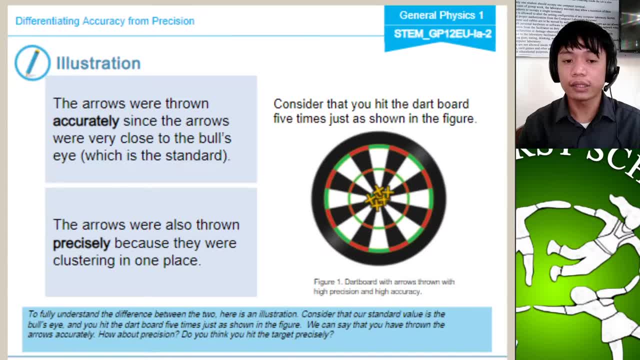 So the arrows were thrown accurately, Since arrows were very close to the bullseye, Which is the. So basically our standard here in playing the dartboard is that the bullseye. So kapag natamaan mo yung bullseye, 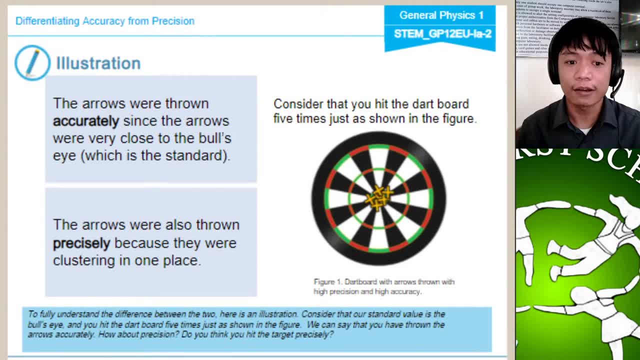 So ang ibig sabihin? nun, you are accurate. Tama ka, okay? So consider that you hit the dartboard five times, just as shown in the picture. So halimbawa, paulit-ulit mong tinamaan yung dartboard. 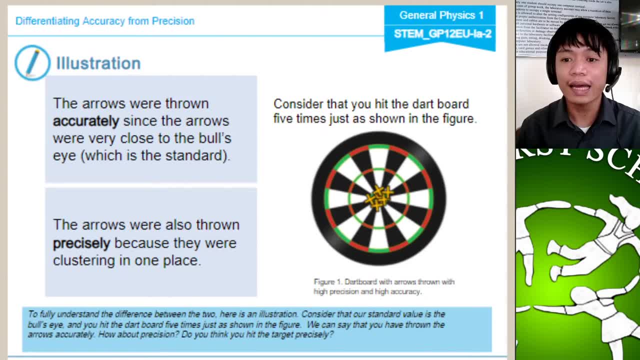 And then The arrows were also thrown, precisely because they were clustering in one place. So ibig sabihin they are grouped mas malapit sila sa isa't isa. So that is precise. So balik tayo ngayon sa repeated measurement na sinasabi: 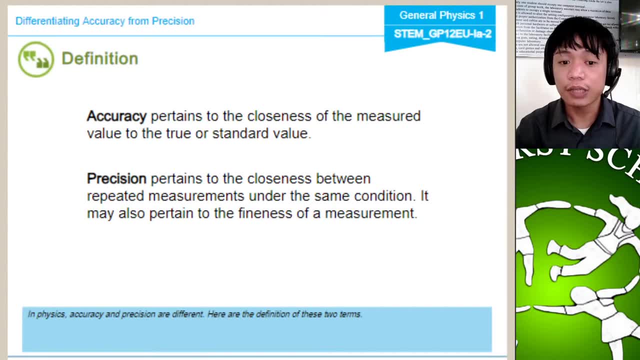 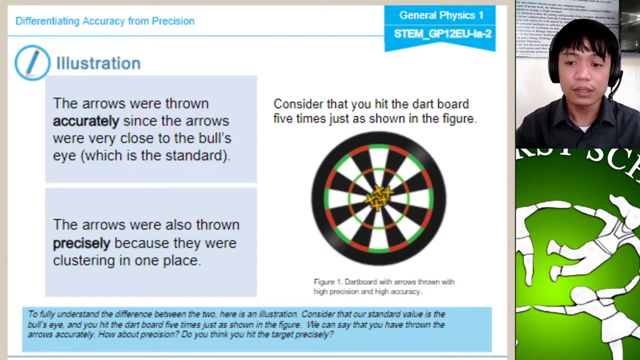 So when we say precision, it pertains to the closeness between repeated measurement. So when we say accuracy, closeness of the measured value to the true value or standard value, So that is their difference. So to fully understand the difference between the two, the illustration has already been drawn. 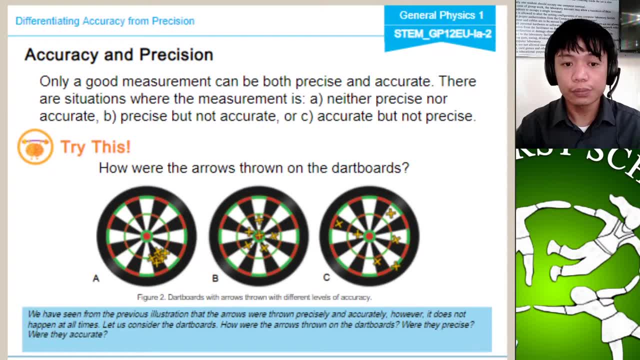 So only a good measurement can be both precise and accurate. There are, There are situations where the measurement is neither precise nor accurate. Precise but not accurate. Pero di namang, accurate but not precise. So try this: How were the arrows thrown on the dartboard? 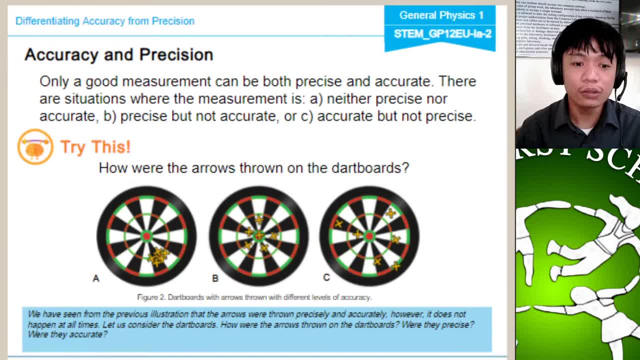 So can you see in the figure A or sa dartboard A na very close yung mga arrows na yun. So ano nga ba yung Masasabi natin, kapag ka very close yung mga arrows, Yung pag hindi siya nakatama sa bullseye, but yung mga thrown arrows or yung mga tinamaan nito is parang magkakalapit sila. 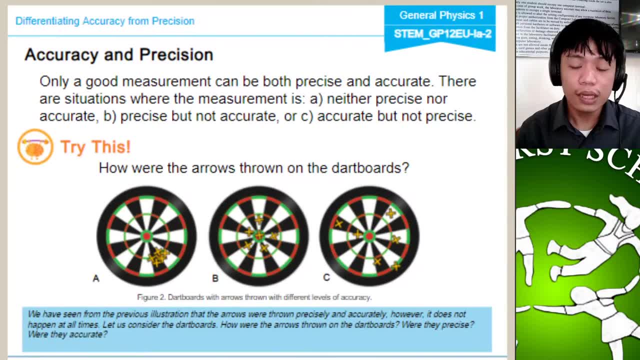 Next see the illustration in letter B. So the illustration there is natamaan mo mismo, Isa mismo, natamaan ng isang arrow, yung bullseye. Ngayon see the difference, since meron tayong anim na arrows doon. 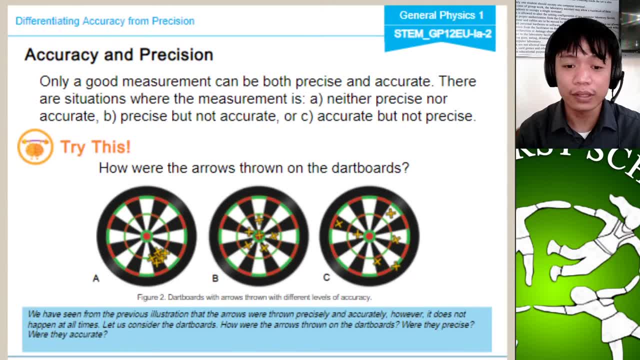 So ngayon, magkakalapit naman yung mga arrows sa bawat isa. So how about yung letter C? So yung letter C, yung mga arrows doon, they are scattered from one place to another. 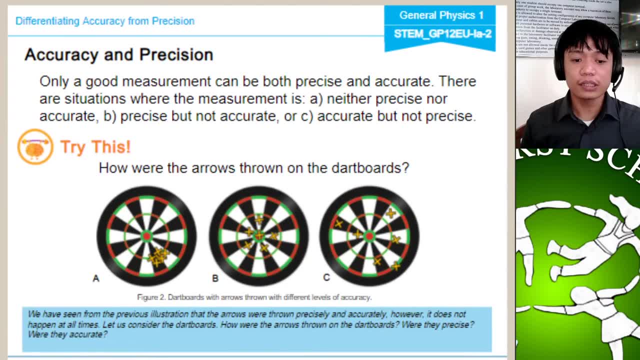 So we have seen from the previous illustration that the arrows were thrown precisely and accurately. However, it doesn't happen at all times. Let us consider the dartboards. and how were the arrows thrown in the dartboard? So let's check. 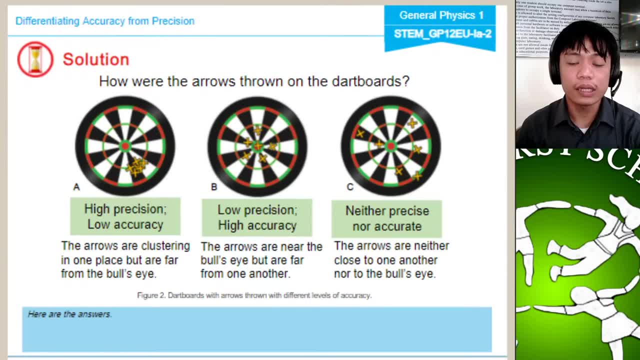 So here is now the illustration of it. Okay, So in letter A it has high precision and low accuracy. So precise yung pagkasabi natin. Or we have high precision, Kasi nga, yung mga measurement mo, yung mga repeated measurement mo, which is the arrows are close to each other. 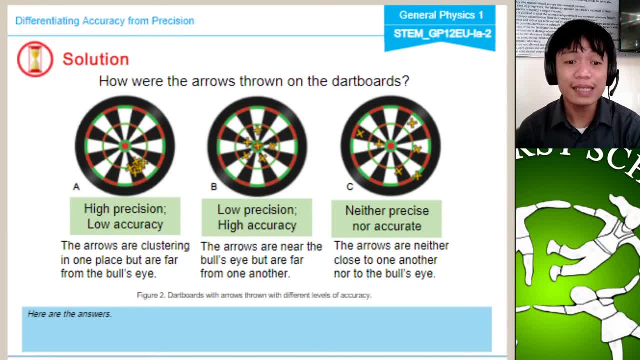 Okay, But it has low accuracy kasi malayo siya sa standard value. Okay, So the arrows are clustering in one place but are far from the bullseye. So that's it. So sa letter B naman. 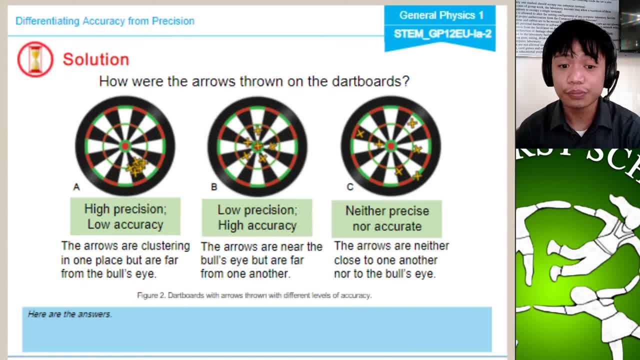 it has high precision. Bakit high precision? Sorry, it has low precision and high accuracy. So meaning to say, sa low precision na yan, yung mga repeated measurement na ginawa mo ay medyong magkakahiwalay. 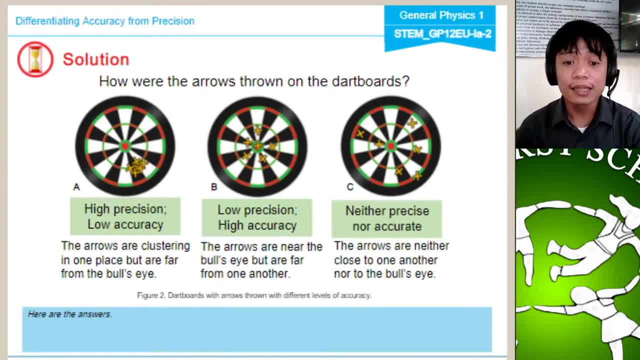 Magkakaiba yung tinamaan nito, Whereas natamaan mo naman yung standard value or yung natamaan mo yung bullseye, which is the standard value. So you have accuracy, Okay. Next, how about sa letter C? 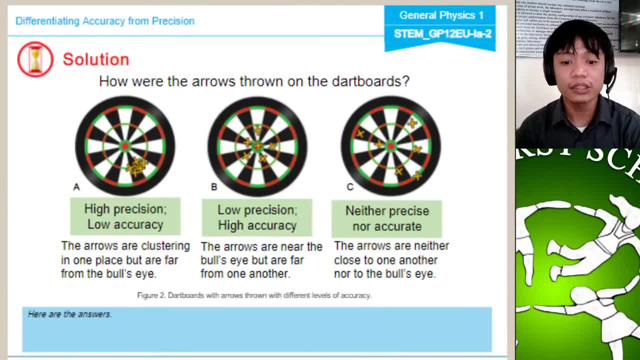 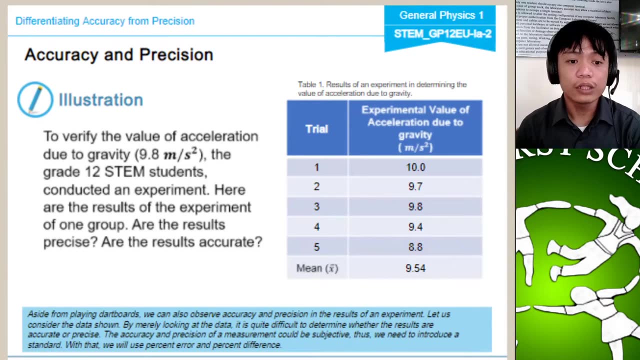 Neither precise nor accurate. So the arrows are neither close to one another nor to the bullseye. So that's it. They are neither precise nor accurate. So to verify the value of the acceleration due to gravity, the grade 12 students conducted an experiment. 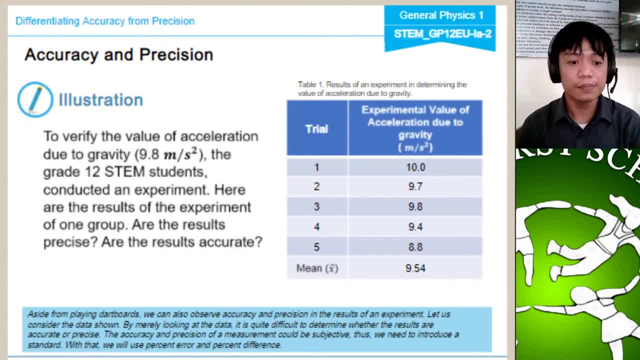 Here are the results of the experiment. Here are the results of the experiment of one group. Are the results precise? Are the results accurate? So here is now the standard, the table 1 that shows the experimental value of the acceleration due to gravity. 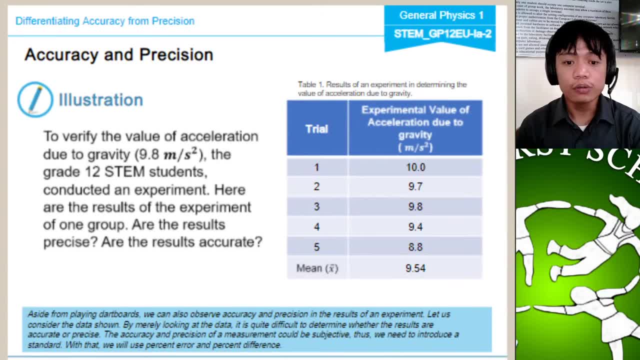 Okay, So we have five trials. So the first trial has 10 meter per second square, followed by 9.7 meter per second square. But the question is: are the results precise and are the results accurate? So what do you think? 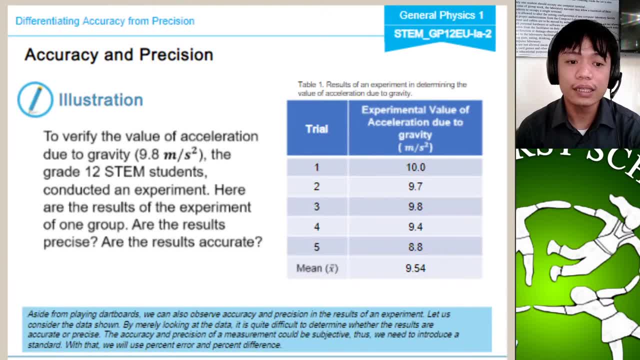 So, basically, the standard value or the acceleration value is the acceleration due to gravity, which is the 9.8 meter per second square. So, based on the presented table, did we met or did we get the 9.8 meter per second square? 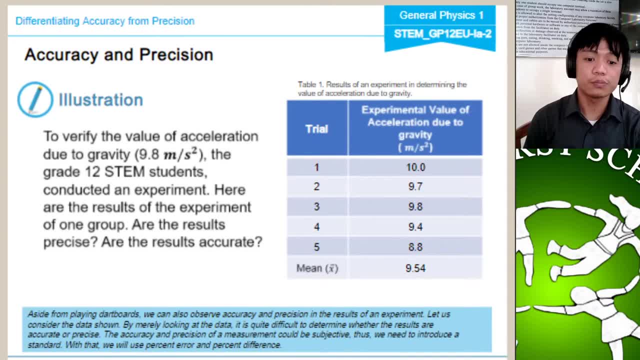 So, aside from playing the dark board, we can also observe accuracy and precision in the results of the experiment. So that's it. So the question is: are the results precise and are the results accurate? Okay, we will know that. 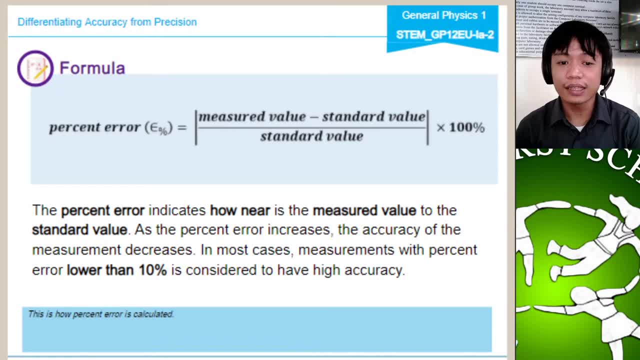 Okay. next, The percent error indicates how near the measured value to the standard value. So meaning to say we have to consider the percent errors. So the formula in getting the percent error is presented now. So percent error is equal to the measured value minus the standard value. 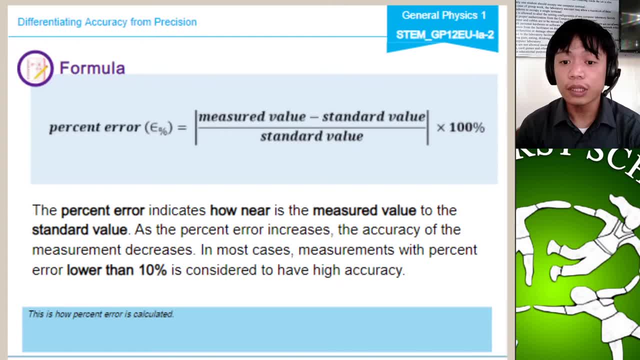 divided by the standard value multiplied to 100. So the percent error indicates how near is the measured value to the standard value. So basically, percent error is pertaining to how close the result of the trial is to the standard value. As the percent error increases, 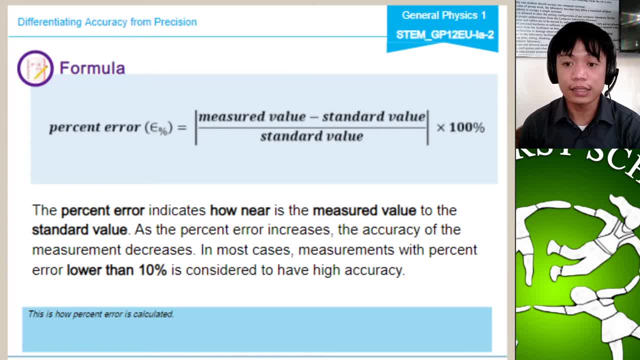 the accuracy of the measurement decreases. So that's it. So you say so that if the percent error increases, the accuracy of the measurement decreases, Because as the value increases or as the percent error increases, meaning to say the accuracy of the measurement is gone. 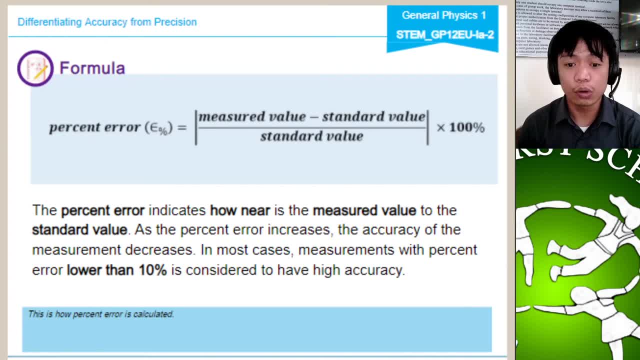 It's like it's getting farther from the standard value. So in most cases, measurements with measurements with percent error lower than 10% is considered to have high accuracy. So basically, if the percent error is lower than 10%. 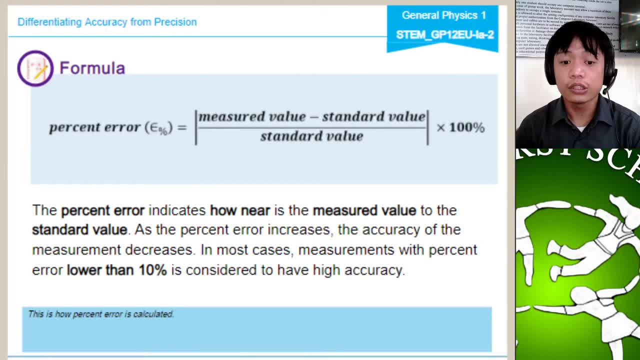 it has high accuracy. So take note of that. If the percent error is lower than 10%, it has high accuracy. So what this means is, as the percent error increases, the accuracy of the measurement decreases. Okay, So next. 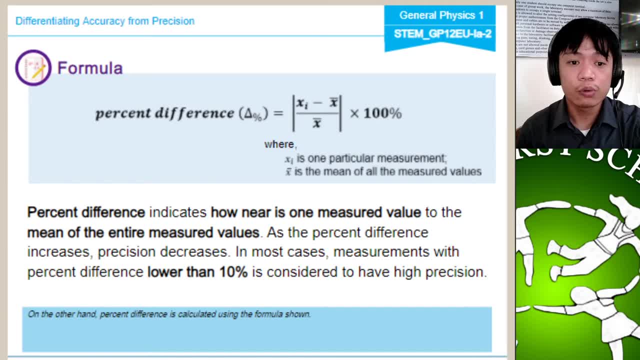 So we have also the percent difference. So when we say percent difference- percent difference is equal to percent difference- indicates how near is one measured value to the mean of the entire measured value. So how do we get the mean? How to get the mean? 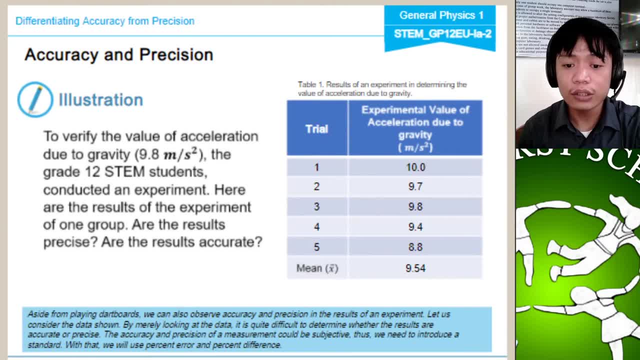 So basically, let's go back here, Let's just add all. let's just add all the values, Okay, The given values, And then, after getting the sum of it, you can just divide it by 5 to get the mean. 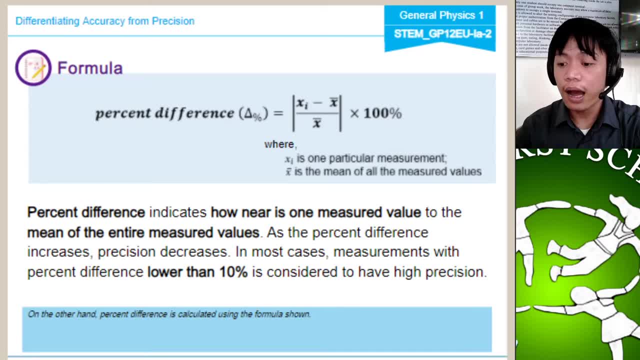 Okay Now so the the formula in getting the percent difference is that we have the. but before that, let's see what is percent difference. So percent difference indicates how near is one measured value to the mean of the entire. 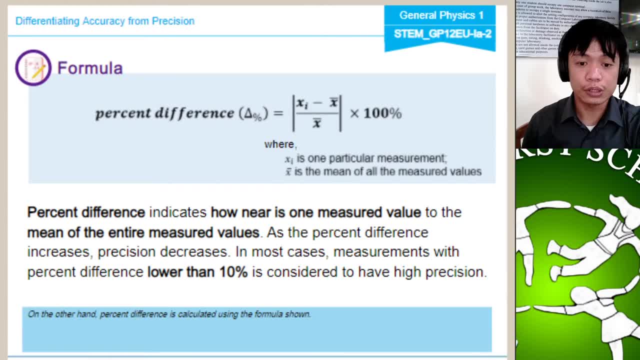 entire measured values. As the percent difference increases, precision decreases. So what is the difference? What is the difference between the two? As the percent difference increases, the precision decreases. So meaning to say, in most cases it is closer to accuracy. 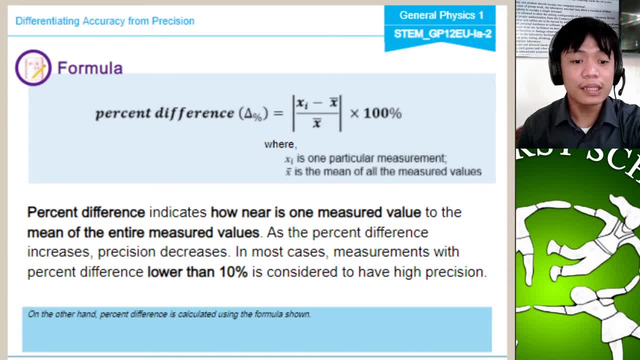 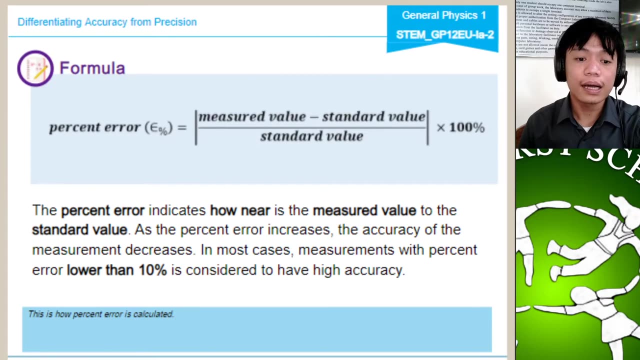 Okay, So measurement with percent difference lower than 10% is considered to have high precision. So meaning to say earlier, in our percent error, if your, if your percent error is lower than 10%, meaning to say you have high accuracy. 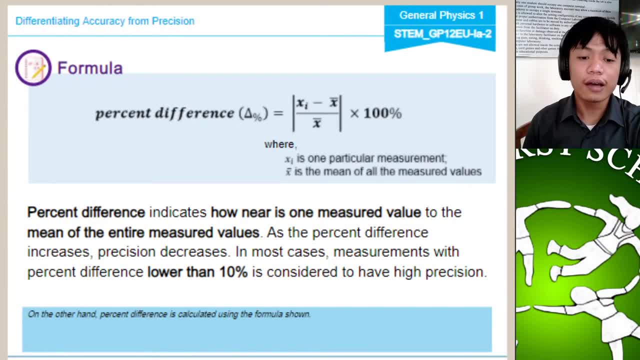 Here in our percent difference. if you have lower than 10%, you have high precision, Meaning to say you are already far from maybe. okay, maybe you are close to accuracy, but you are, you have a high precision. 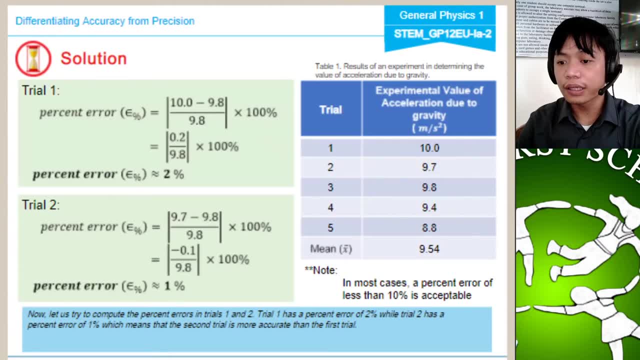 So, for for you to understand more regarding this, we have this. ah, we have this solution. So, trial: one Percent error is equal to 10,, which is the given value, minus 9.8,, which is the standard value. 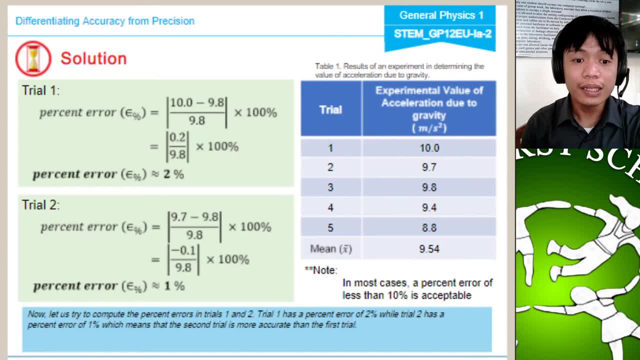 times 100.. So we did get 2%. So meaning to say percent error is 2%. Kapag ka 2%, yung percent error. is it precise Or is it accurate? Does it have a high precision? 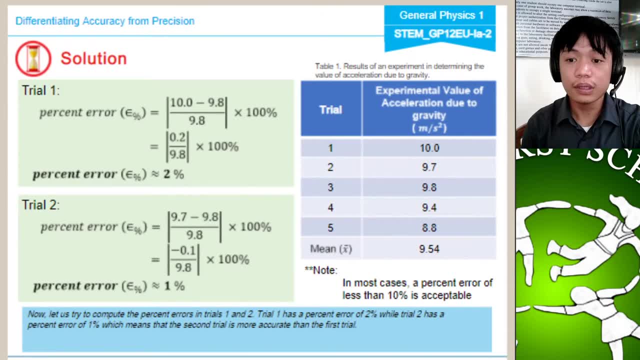 Or does it have a low ah precision, Or mataas ba yung accuracy Or mababa ba yung accuracy. So take note na kapag mababa yung percent error, which is the 2% mataas yung accuracy level, 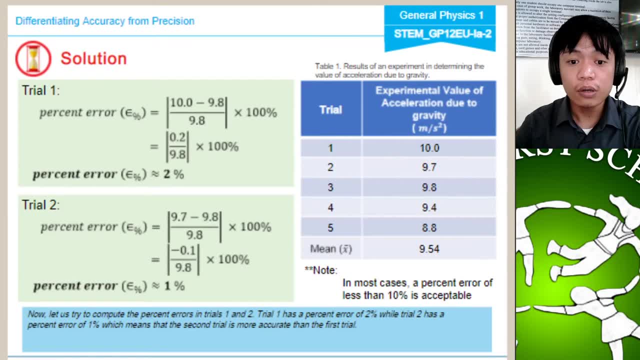 ng inyong experiment. So halimbawa, neto is: we have 2%, So the the given values is, values here is 2%. So kapag ang naging ah like, for example, the given here is: 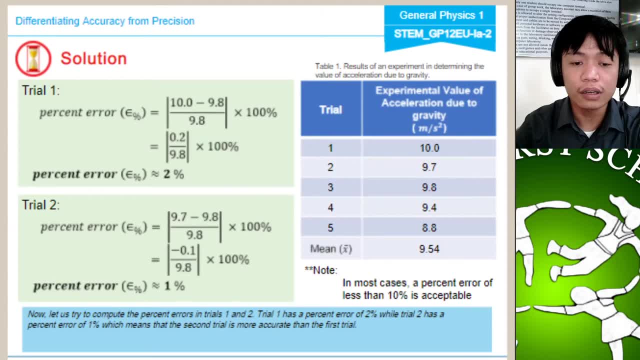 the experimental value of the acceleration due to the gravity in trial one is 10% minus the standard value, which is the 9.8.. So malapit lang naman, kasi ang 9.8,. ah, ang 10 sa 9.8,. 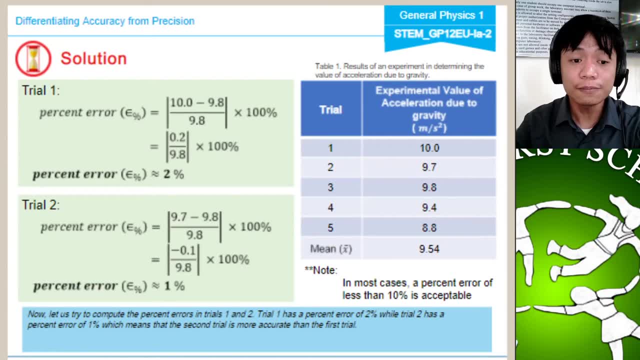 which is your standard value. So meaning to say the percent error is 2.. So mababa sya, So mataas yung accuracy level neto. So what about in percent? ah, dito sa trial 2?. 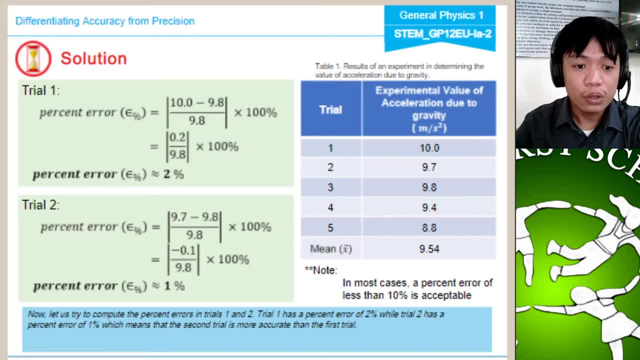 Okay, See the difference. So alin ba ang mas malapit sa 9.8? Yung 10 ba na first trial Or yung 9.7?? Okay, let's see. Percent error is equal to 9.8 minus 9.7 minus 9.8 divided by 9.8, multiplied to 100.. 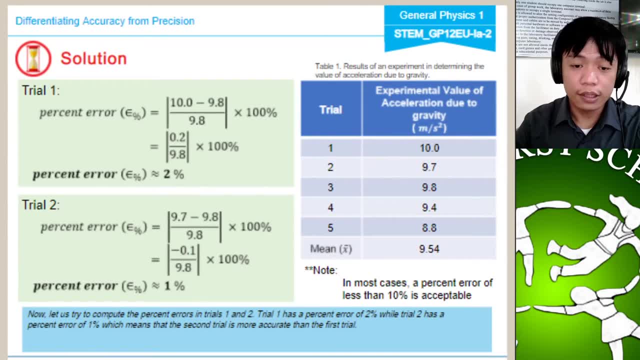 So we got 0.1 divided by 9.8.. So the percent error is equivalent now to 1%. And take note: kapag mas mababa, kapag mas mababa yung percent error, it has high accuracy. 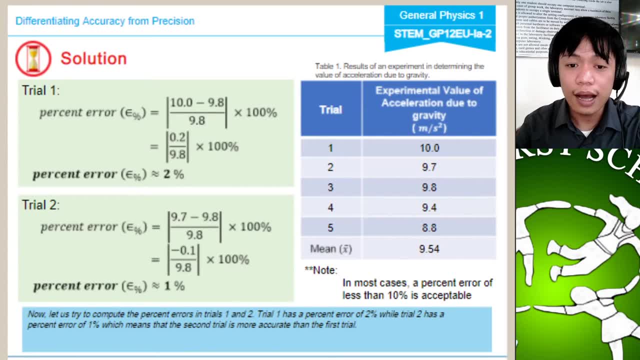 So take note, tignan nyo dito sa ating, ah, sa ating table. Okay, So yung yung ating acceleration due to gravity is 9.8.. Right, So ang 9.7 ay malapit sa 9.8.. 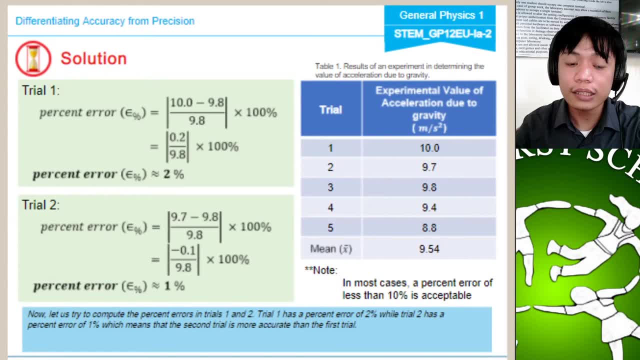 Okay, So parang ang percent error lang niya is 1%, So ah, mas malapit siya sa accuracy. Okay, So take note class dito na if the percent error is, ah, lower than 10%, it has high accuracy. 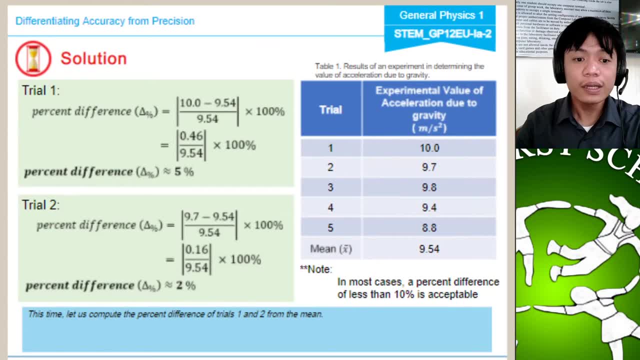 Okay, So let's proceed. So what about the percent difference? So the percent difference is equal to 10,, which is the given value, Minus 9.54,, which is the mean. Okay, Yun, yung mean. 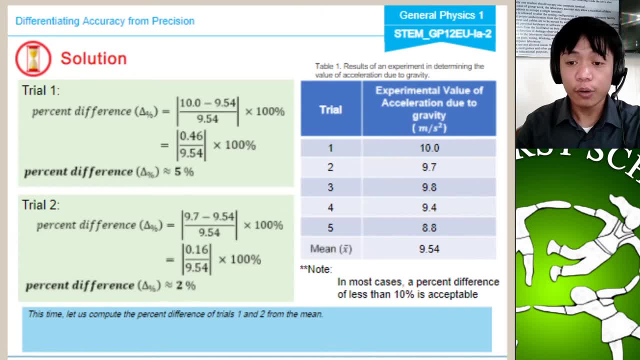 Okay, Divided by 9.54, which is the mean times 100.. So we did get 5%. So take note that 5% is also ah medyo. it's considered as accurate, pa rin. 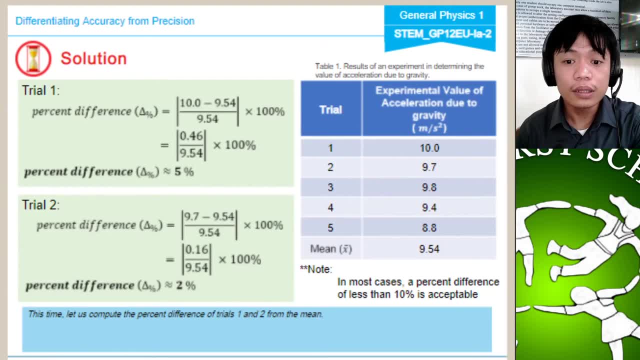 So medyo mas accurate pa rin siya. So take note. So take note na ang 10 is malapit pa rin siya sa 9.8.. Now, what about the percent difference in trial 2?? So mas malapit ang 9.7 sa 9.8.. 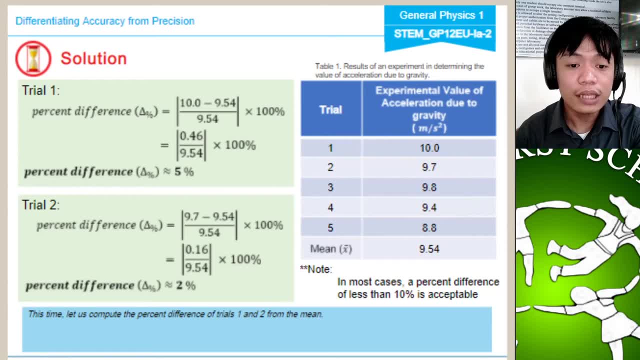 But let's see. So 9.7 minus the 9.54 divided by 9.54 times 100 is equal to 0.16 divided by 9.54 times 100. So we did get 2%. 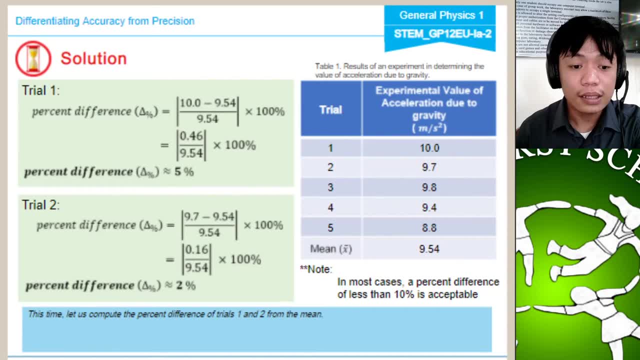 Meaning to say mas accurate na naman yung trial 2.. So paano kapag ka ang ating trial 3 ang gagamitin? So basically, kapag percent difference ang gagamitin natin 9.8 minus 9.54 divided by 9.54 times 100 is equal to 1.2.. 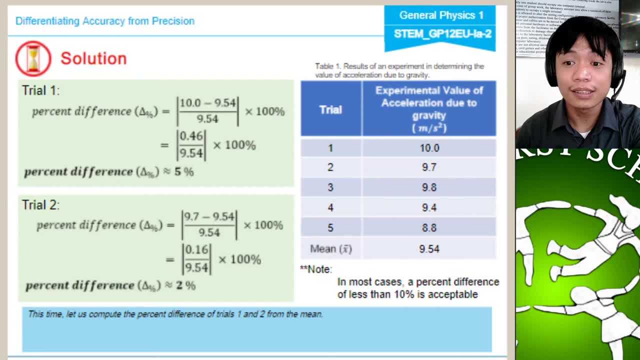 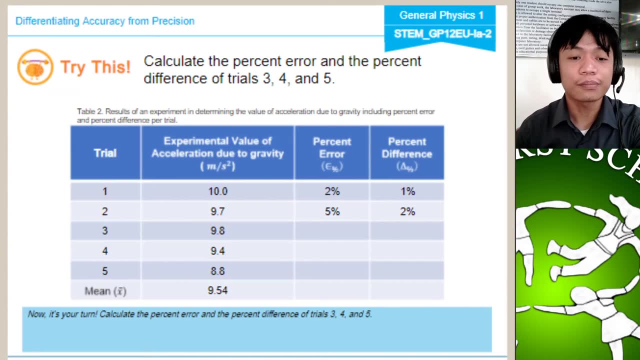 is equal to what? so answer that later on. so let's try this. okay, calculate the percent error and the percent difference of trials three, four and five. so tapas na tayong nag-identify ng percent error at percent difference the trial one and two. so take note of our, take note of our formula. so 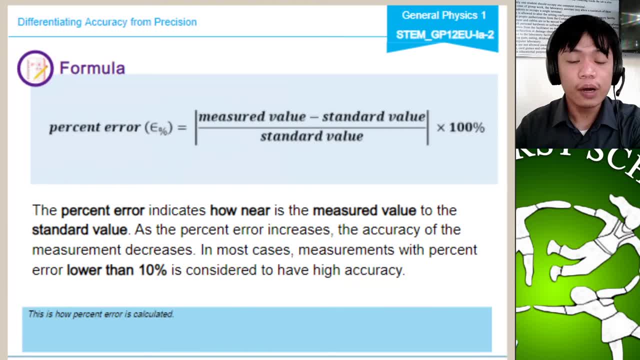 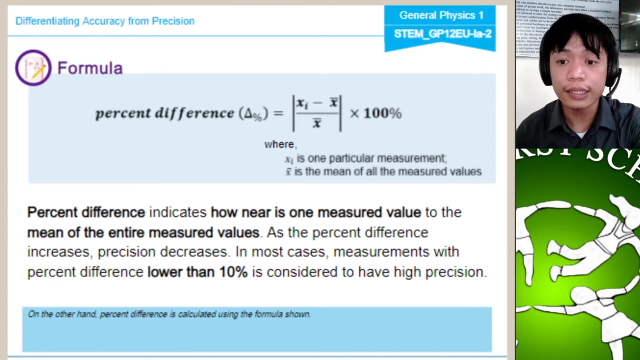 balik tayo sa ating formula. okay for you to understand the formula of percent error. percent error is equal to measured value or the given value minus the standard value divided by the standard value multiplied to 100. next percent difference is equal to the given value or the initial value or the measured value minus the. 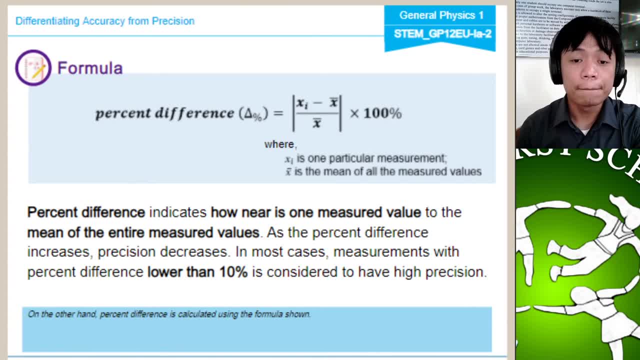 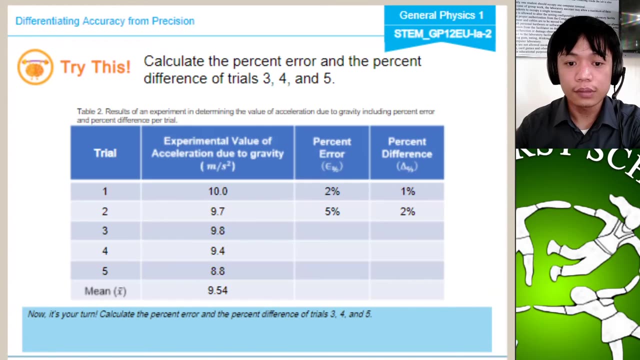 mean of the given values, minus, I did, divided by divided by the mean times 100. so let's do this. I'll give you, I'll give you time to finish that. so for nine point eight, nine point four and eight point eight, you should finish that and I will message me if you already. 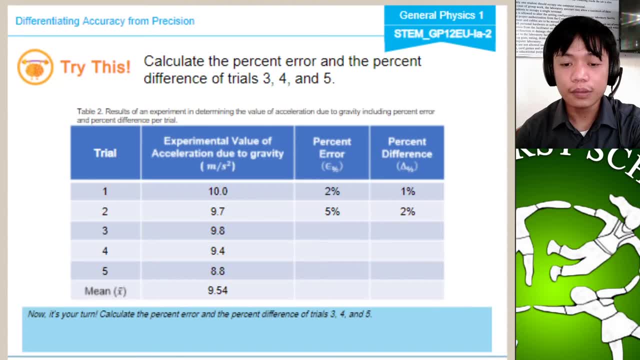 finish that para at least. uh, mamayang, alas, dapat natapos in mamayang 820. okay, 820, dapat natapos. sorry, dapat. uh, nine o'clock, tapos nyo na. okay, nine o'clock. tapos nyo na yung number three, four, five. 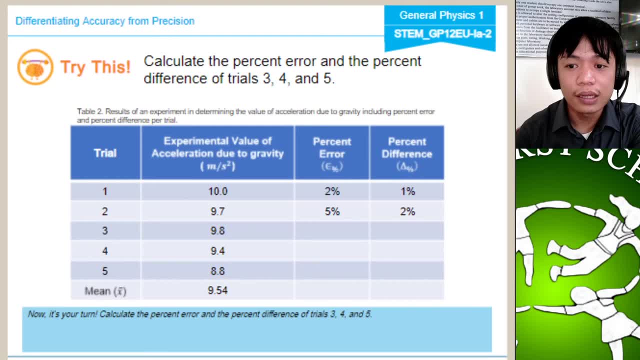 trial. So ano, kaya The question is yung fifth trial natin. what do you think? Okay, Is it high accuracy ba siya? Accurate ba yung kanya. How about number four? Is it high accuracy, Does it? 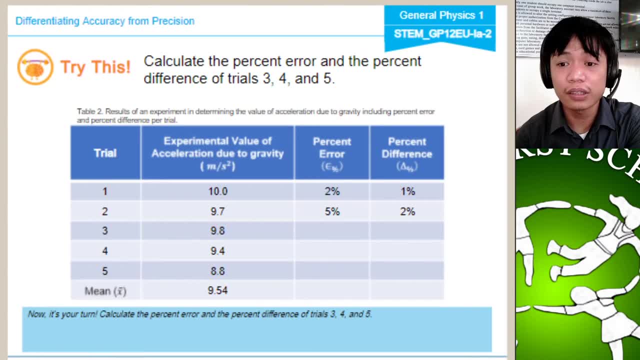 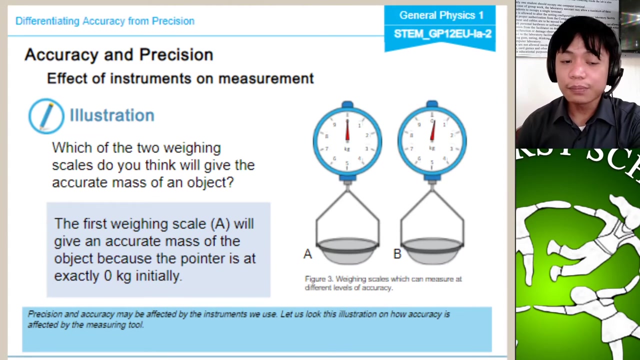 have high accuracy. How about yung trial number three? So I'm going to check that later on. So now you can screen capture that and I'll be waiting for your answer at exactly nine o'clock today, Okay. Next, The accuracy and precision: okay. effect of instrument in measurement. So 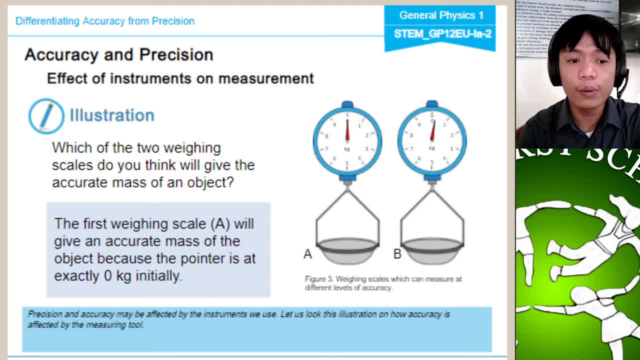 what do you think? Which of these two weighing scale do you think will give the accurate mass of an object? So meron tayong dalawang kiluhan dito. Okay, Now the figure three is weighing scale which can measure at different level of accuracy. So what do you think The first weighing scale, A, will give an accurate mass of object, because the pointer is at: 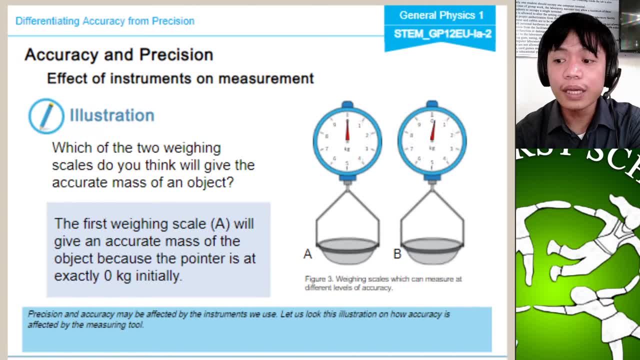 exactly zero kilogram initially. So basically the standard value for the kilogram is zero. So syempre ano bang bang pipiliin mo kapag pupunta ka sa palengke at mamimili. Syempre on nakatapat sa zero because it is, it is the standard value. okay, So kapag nga nakita mo medyo tagilid yung kiluhan syempre medyo magkakaroon ka nalang agos pa. Okay, Now you are doing the second weighing scale to get the exacteur on the scale Madating as possible. go ahead with the second weighing scale. potatoes. 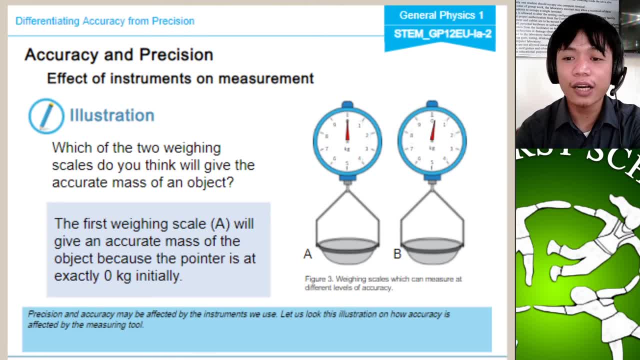 yung kiluhan. syempre medyo magkakaroon ka nalang agam-agam tungkol dito. Kaya ang gagawin mo or ang ginagawa ng iba is medyo sinusobrahan nila yung value. 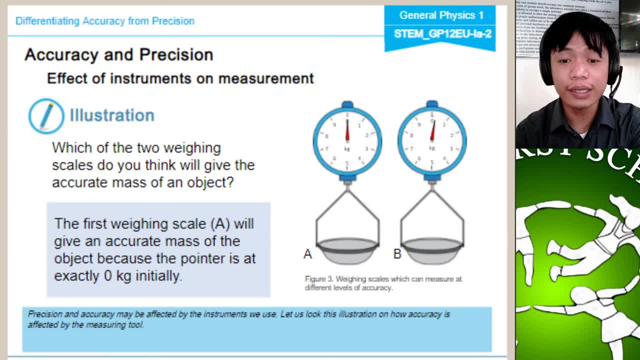 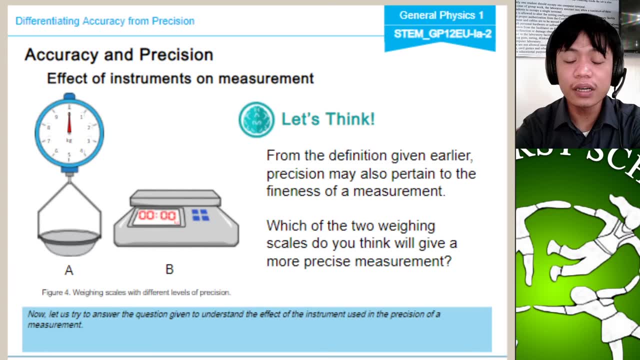 or ginagawa nilang accurate, or nakatapat talaga sa zero yung value. So next, From the definition given earlier, precision may also pertain to the fineness of the measurement. Now the question is which of the two weighing scale do you think will give a more precise measurement? 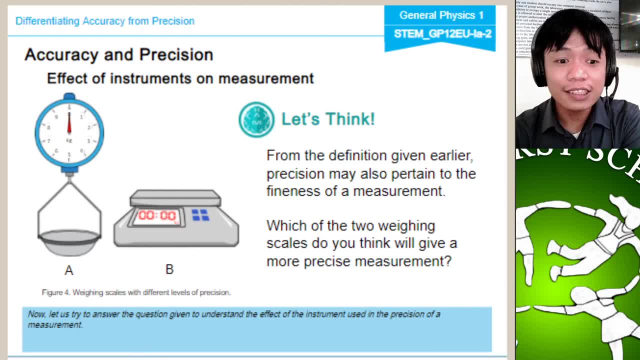 So yung kanina, yes, sa ating letter A, which is the standard weighing scale, Meron tayong standard and digital weighing scale. So we have a standard and digital weighing scale. From that two object or, true, from that two measuring instrument, which of these two are more precise? 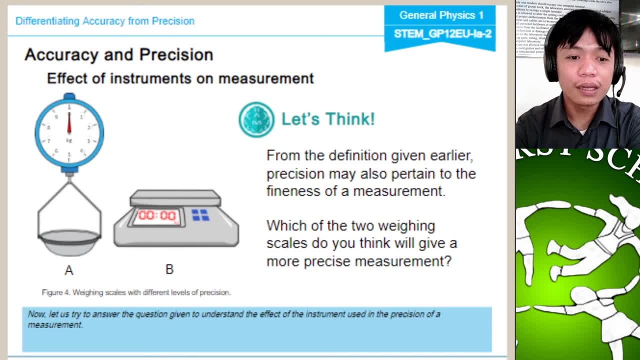 Okay, more precise. So I'll give you five seconds to answer: A, A or B, 5,, 4,, 3,, 2, 1.. So the correct answer is letter B. Okay, so that's it. 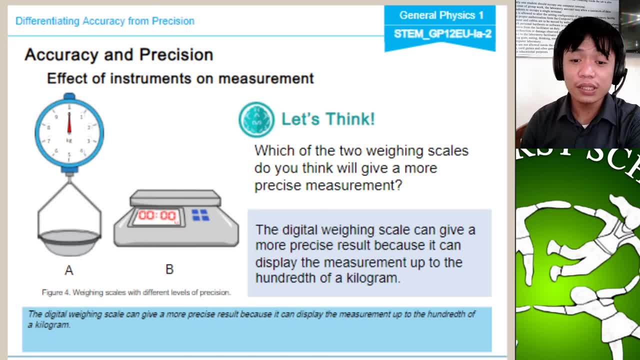 So the digital weighing scale can give a more precise result because it can display the measurement of the hundreds of kilogram. That's it Kasi. meron siyang repeated values. Okay, meron siyang repeated parang measurement. Dinidisplay niya parin yung. 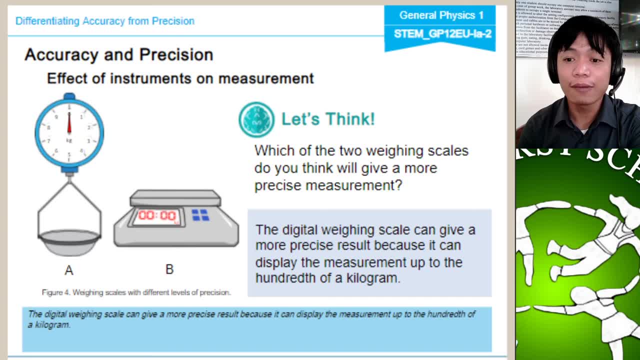 Halimbawa, we have 1 kilogram, 1.8.. So yung 8 doon is, halimbawa it's a mass, okay, Or what do you call this E-value? also, Parang it is a repeated measurement. 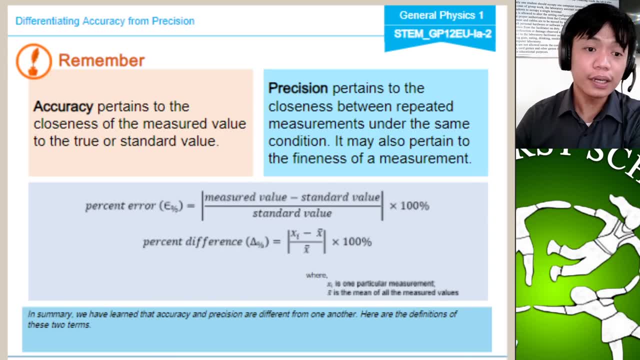 So take note or remember. accuracy pertains to the closeness of the measured value to the true or standard value. Next, precision pertains to the closeness between repeated measurement under the same condition, and it may also pertain to the fineness of the measurement.